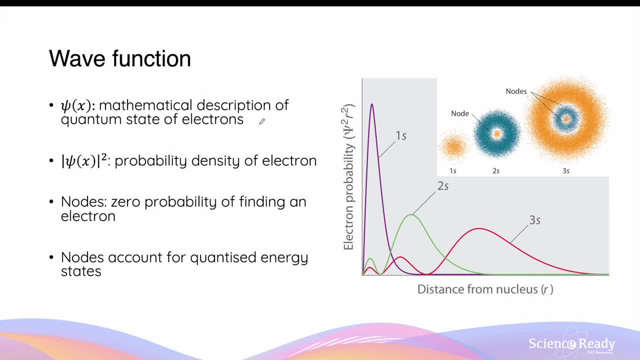 Schrodinger's model of the atom is accompanied by the wave function. The wave function is a mathematical description of the quantum state of electrons. I'll discuss what I mean by quantum state in a moment. The relevance of the wave function to this probabilistic model is that 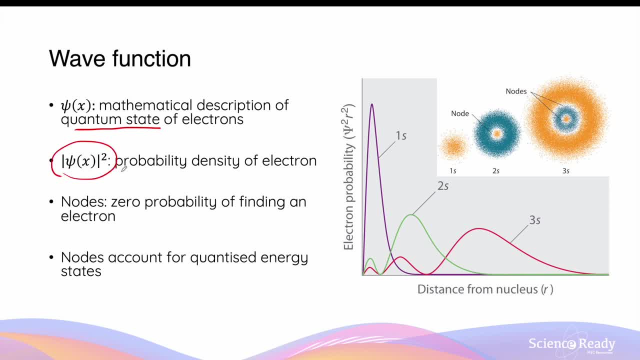 when you square the wave function. it provides you with an equation that describes the probability density of the electron, which is what we saw in the orbital diagram earlier. This graph provides a visual representation of the square of the wave function, or in other words, the electron probability of three different 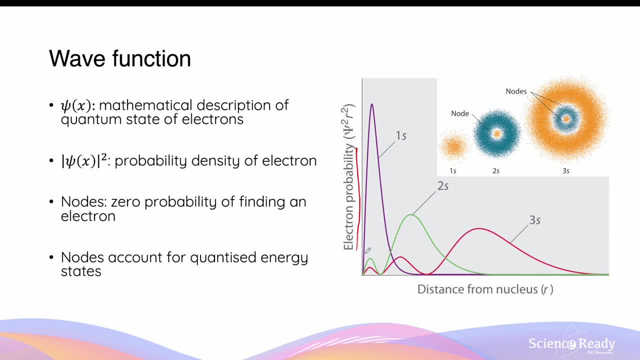 orbitals, The 1s, 2s and 3s orbital. You can see that the probability is not constant. It changes throughout each orbital and the probability is also different between different orbitals. This diagram here is a direct comparison of what the probability density. 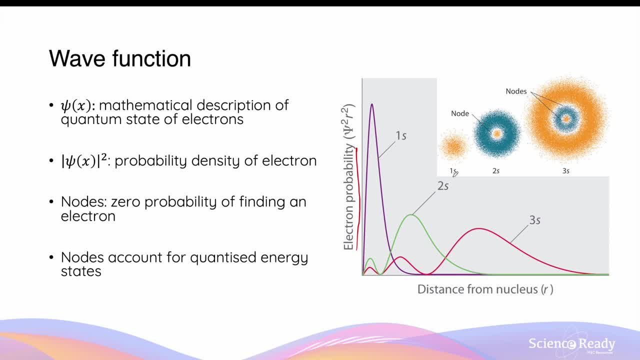 diagram looks like in relation to the graph shown. The 1s orbital is surrounded by the 2s orbital and the 2s orbital is further surrounded by the 3s orbital. You can clearly see that between the orbitals there's a white concentric region where you cannot find any electrons. 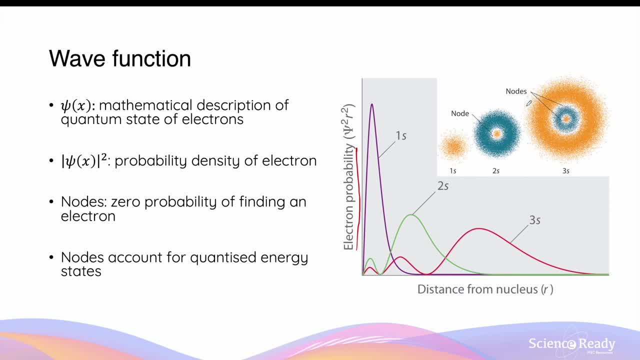 These are known as the nodes in Schrodinger's atomic model. Nodes are regions where there's a zero probability of finding an electron, and they account for the quantization of the energy states of electrons that was described earlier in Bohr's model of the atom. 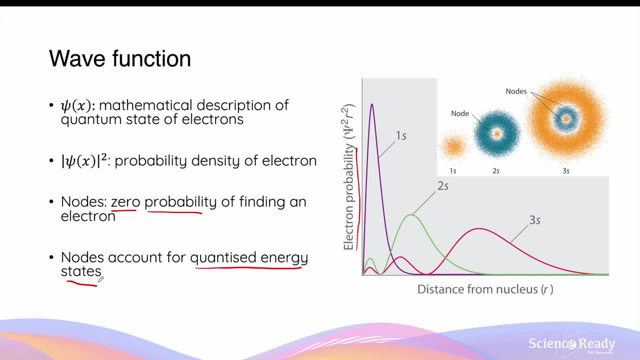 Quantization of energy states mean that the energy of electrons orbitals must be a multiple of a specific value. The nodes are forbidden areas where you cannot find electrons, as the energy in these regions are not a multiple of that small value, Quantum numbers are. 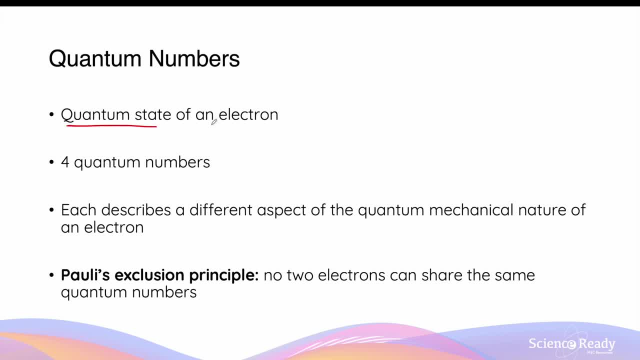 associated with Schrodinger's atomic model, as they describe the quantum state of an electron. There are a total of four quantum numbers. Each quantum number describes a different aspect of the quantum mechanical nature of an electron. Each electron will have four quantum numbers. According to Pauli's exclusion principle, no two electrons can share the same quantum number. 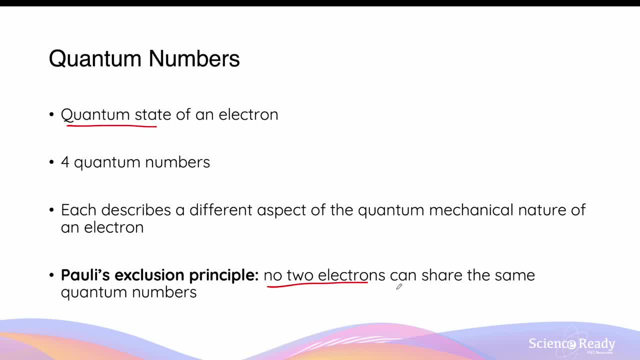 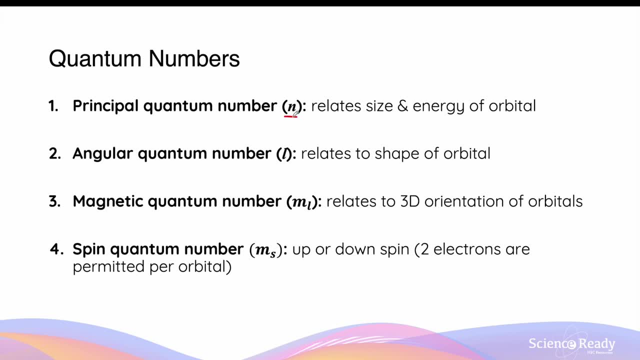 That means in a given atom, every electron has its unique set of four quantum numbers. The first quantum number is known as a principal quantum number, denoted by n, and this determines the size of the energy of the orbital. so whether it's 1s orbital, 2s orbital or 3s orbital, 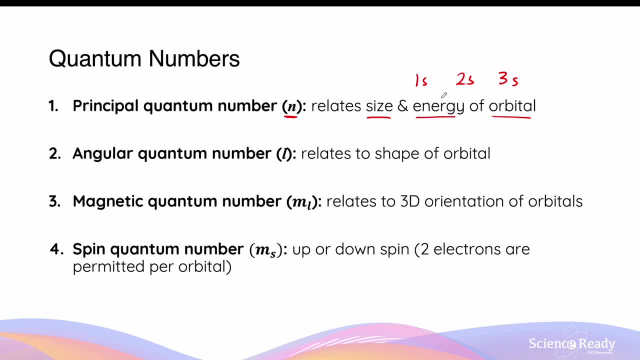 The size, the energy is also related to the distance of the orbital away from the nucleus. The second quantum number is known as the angular quantum number, denoted by the letter L. This relates to the shape of the orbital. We'll have a look at what this- we'll have a look at-. 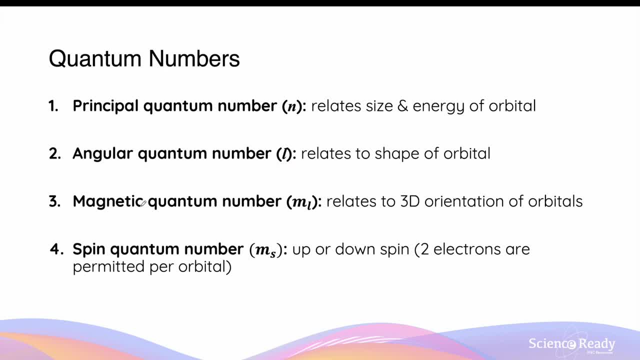 we'll have a look at the different shapes in a moment. The third quantum number is the magnetic quantum number, or ML. relates to the orientation of the orbitals. The fourth quantum number is the spin quantum number, or MS. This determines the magnetic spin property of electrons. The spin of the electron can either: 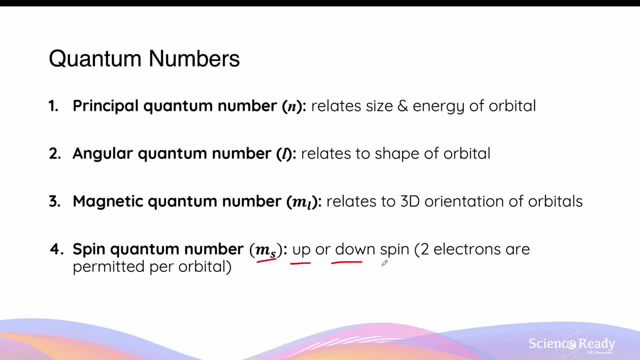 be up or down, and in each orbital there can be a total of two electrons. and each orbital there's a maximum of two electrons, where one electron will take the up spin and the other will take the down spin. The size energy of orbitals increases with its distance from the nucleus. 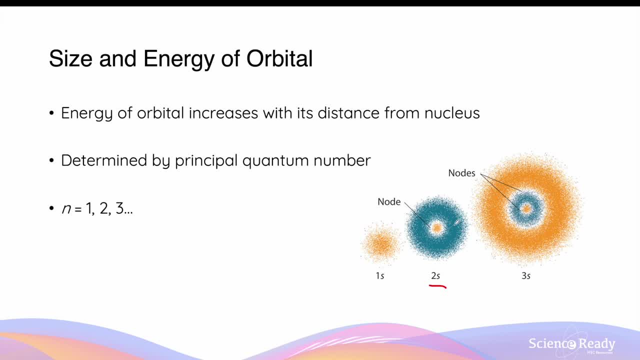 So 2s orbital is further away from the nucleus and therefore has a high energy compared to the 1s orbital. and 3s orbital is further away than the 2s orbital. therefore it has a greater energy compared to 2s orbital. The energy of the orbital is determined by the principal quantum number. 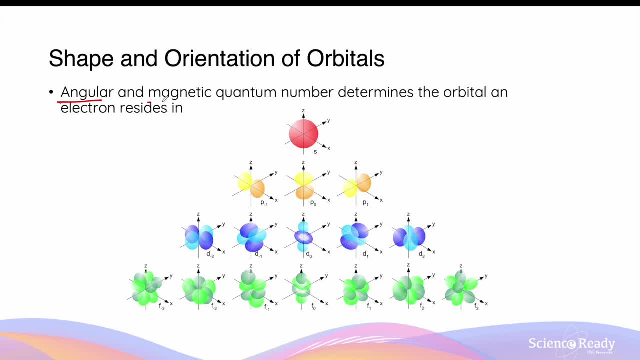 n. The second and third quantum numbers, or the angular and the magnetic quantum numbers, determine the shape of the orbital and the orientation of the orbital. So far, we've only looked at the s orbital. however, orbitals can take on different shapes, such as p orbitals, d orbitals and f orbitals. The second quantum number determines the shape of the. 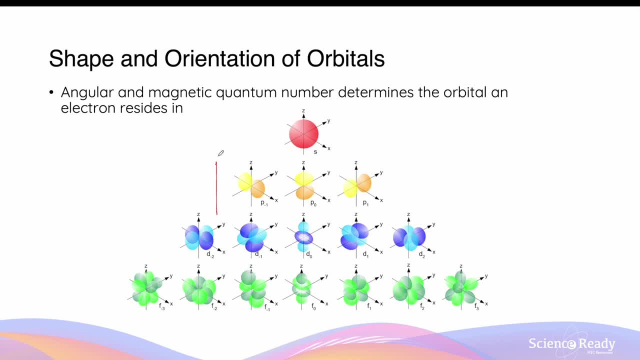 orbitals. each electron will be found in Amongst each type of shape of orbital. you can have different orientations, and this is determined by the third quantum number, the magnetic quantum number. For example, the p orbitals can take on three different orientations. where the plane is, 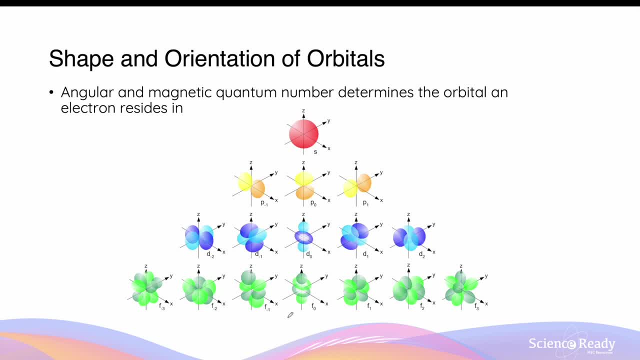 located, and the f orbitals can take on seven different orientations. This concludes the video on schrodinger's atomic model.